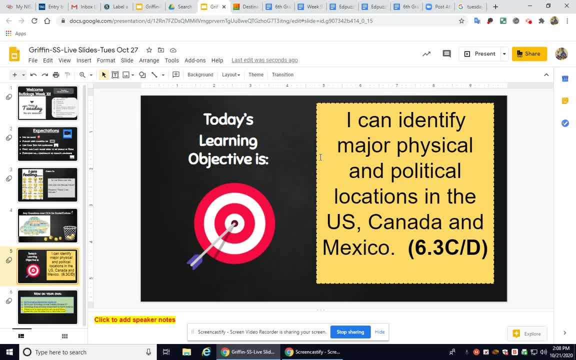 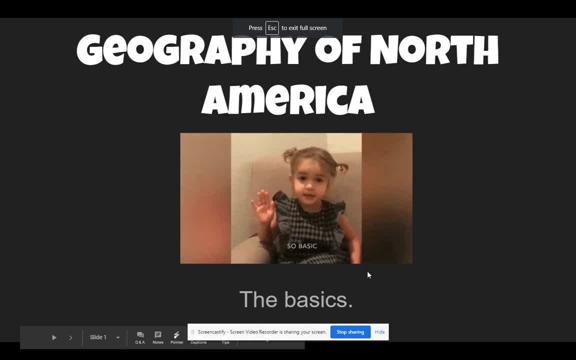 So remember, we're going to focus on these three countries in the North American continent. So for today's lesson we will look at the geography, Geography of North America, the basics. Okay, first things first. North America is a continent. 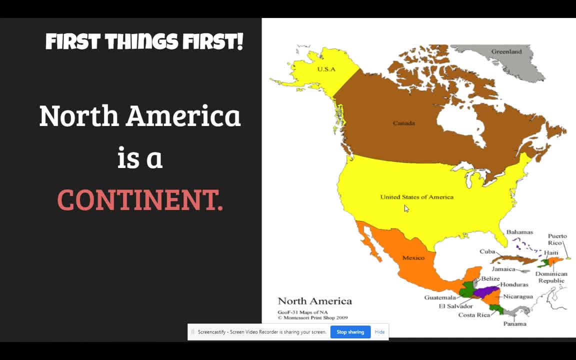 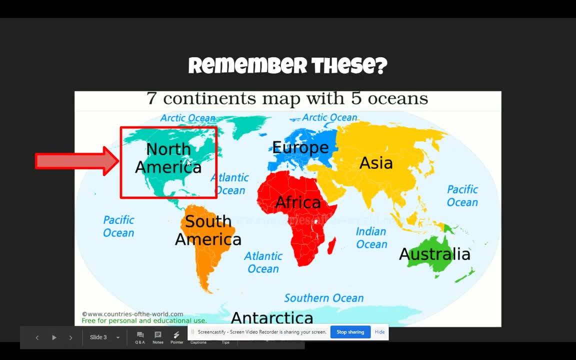 Alright, the three countries we're looking at is Canada, the United States of America and Mexico. Remember, North America is a whole continent. Next, we have seven continents, Okay, and remember, we have five major oceans. Okay, the continent we're going to focus on today is North America. 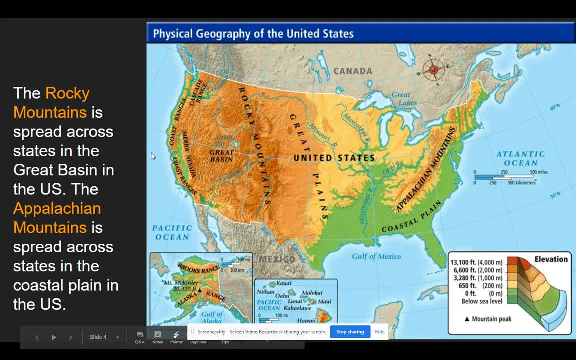 So the physical geography of the United States. This will help you in your Schoology assessment. We are going to look at the Rocky Mountains. Okay, spread across the states in the Great Basin in the US, if you guys see right here. 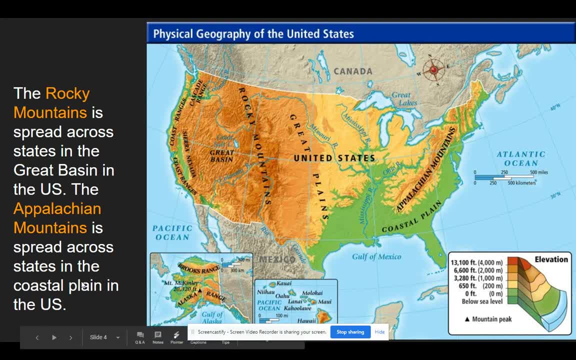 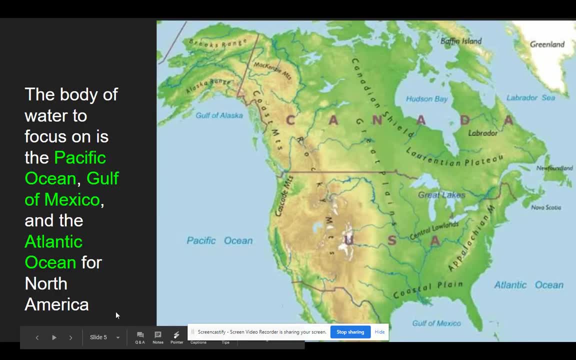 Next, we're going to look at the Appalachian Mountains, which is spread across states in the coastal plain of the US, Alright. Next we're going to look at the body of waters around North America, The main ones we're going to focus on. 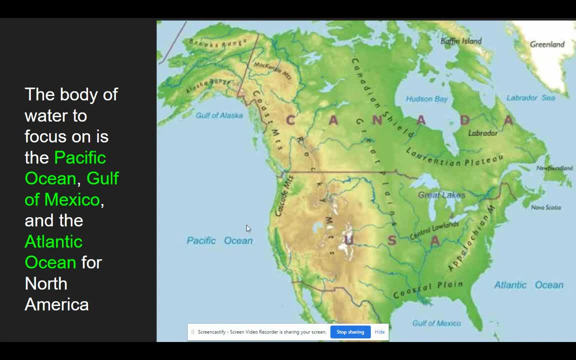 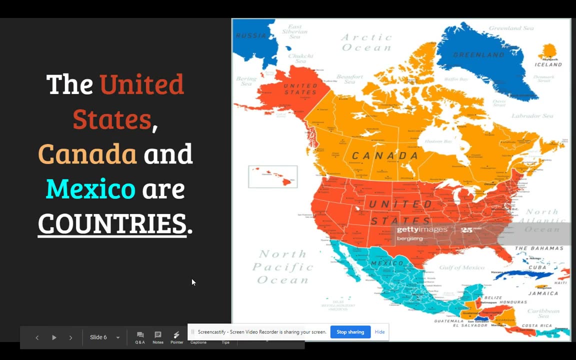 on is the Pacific Ocean, the Gulf of Mexico and Atlantic Ocean. okay, those are the three bodies of waters that we're going to focus on from North America. next, the countries that we're going to focus on in North America is the United States, Canada and Mexico, and if you guys see later on in the slideshow, you see 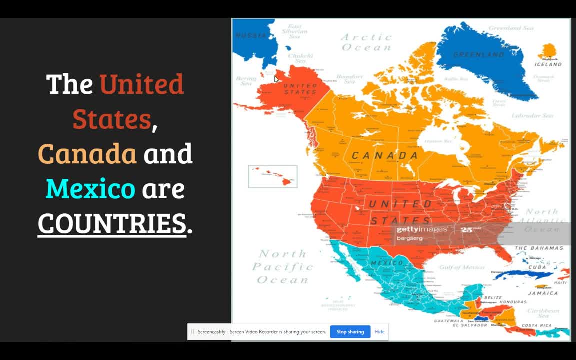 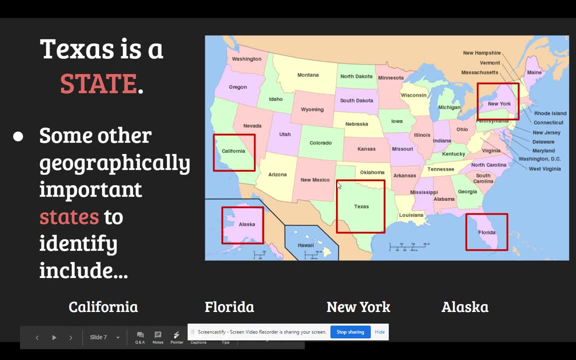 this is part of the United States. this is Alaska. this is Alaska up here. next we're going to look at the states of the United States. okay, remember, Texas is a state. we have a total of 50 states in the United States. okay, and if you see, 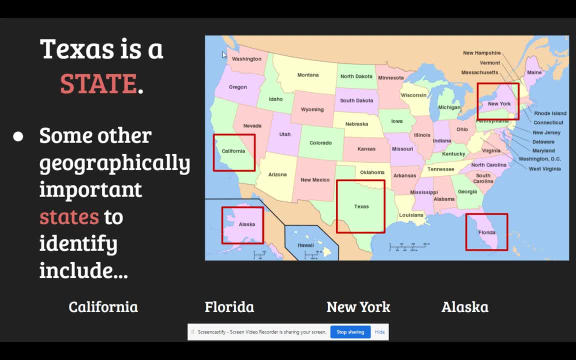 right here. Alaska is right here, but it is on a Northwest part of the maps when we, when we spread out the whole continent of North America and you guys will see that okay. so some of the other geographically important states to identify is California, which is right here. on our west coast again, we have Florida. 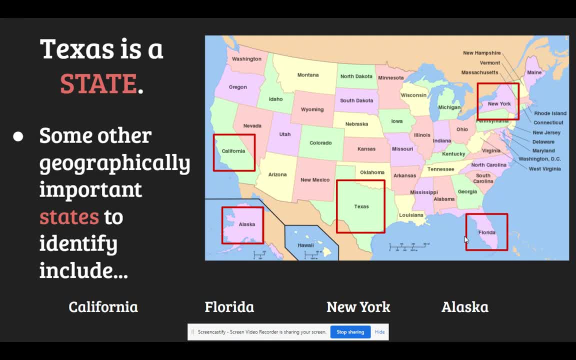 that's over here in our southern east coast, in our coastal plains area. okay, we also have New York, which is on the top east, is our east coast, one of our biggest cities in the United States. and then we have Alaska, which I said is on a Northwest part near Canada. again, Alaska is on the north, is actually Northwest of. 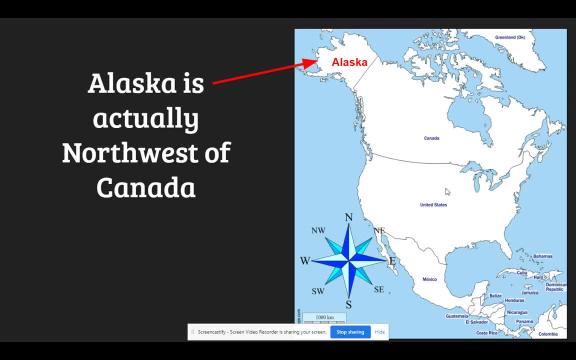 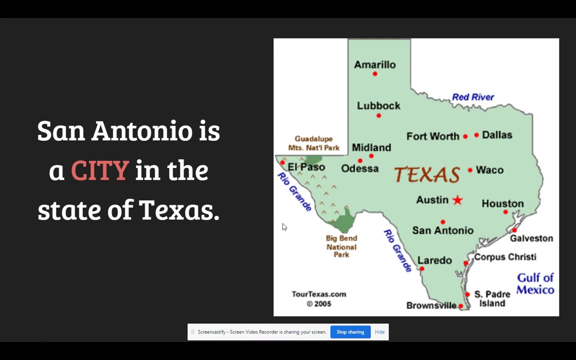 the United States. ok, so we can just make sure you have information coming out. you got which Alaska, which Alaska is part of the United states. alright, if you make sure when you're looking at map keys you also look at the compasses. ok, if you see us Northwest of Canada, in the States, we 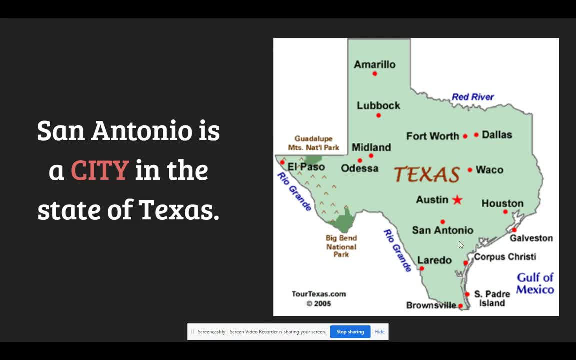 have cities that are in each of the 50 states in the United States and where we're located at. we live in San Antonio, Texas, which is a City of Texas, and if you see we're stars at, that is Austin, which is our capital city of Texas. we live in San Antonio, Texas, which is a City of Texas, and if you see we're experi as that, that is Austin, which is ourénomina attributes. we know what we're looking at, which we can okay there to come back into the form, the west, and we'll have more details in a minute with this talk, but right now we'll take the next slide quejo a look for better sense of the personella form. a long time now. 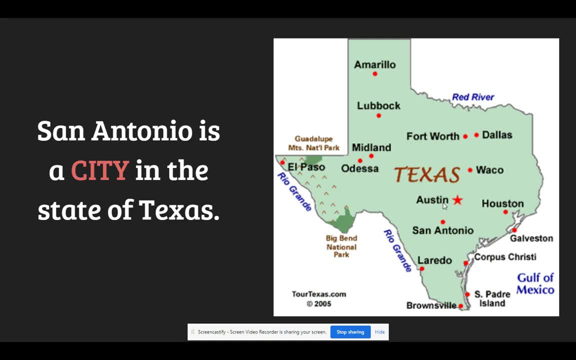 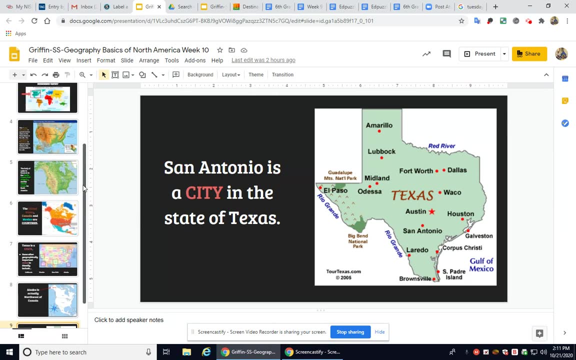 city of Texas and if you look at maps in each state, this the capital city and each state has a star on it. so make sure you guys keep that in mind, okay, so for today I want to show you guys your Schoology assessment and some things that will actually help you guys out. okay, so here's a look at your Schoology. 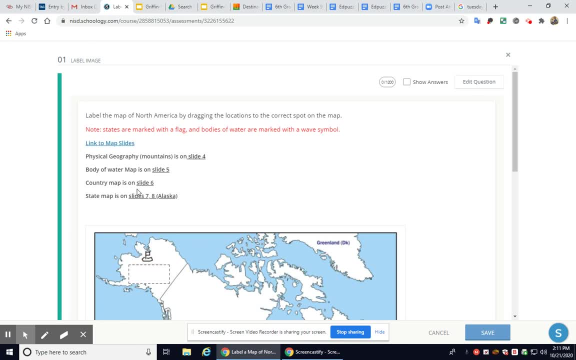 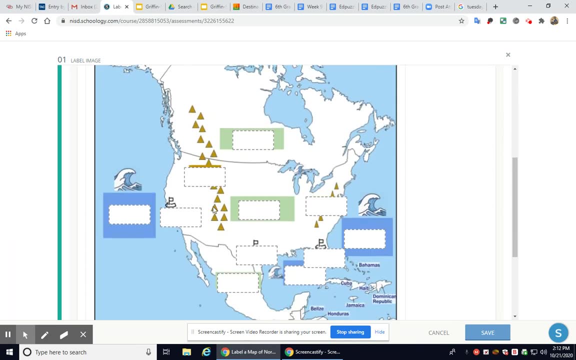 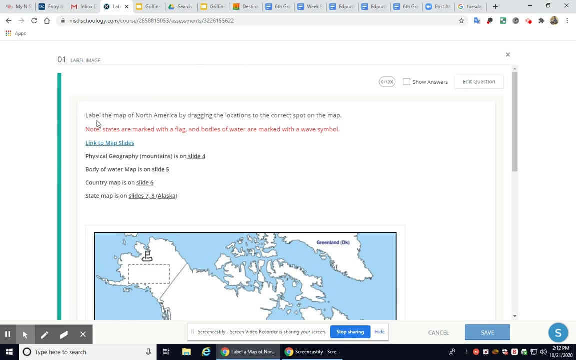 assessment. all right, please read the question set up. this is really going to help you guys out. okay, as you guys see, you have the North American continent, you have dragon drops. okay, you make sure you place these in the correct places. so, first things first, label the map of North America by dragging the locations. 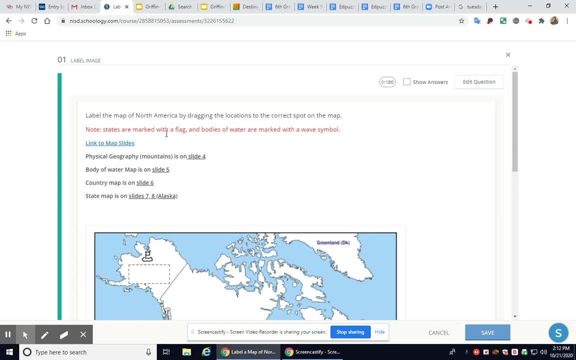 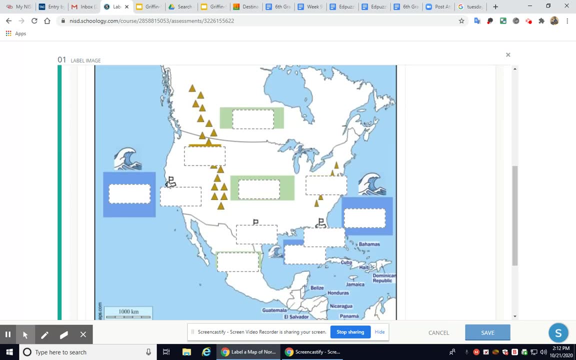 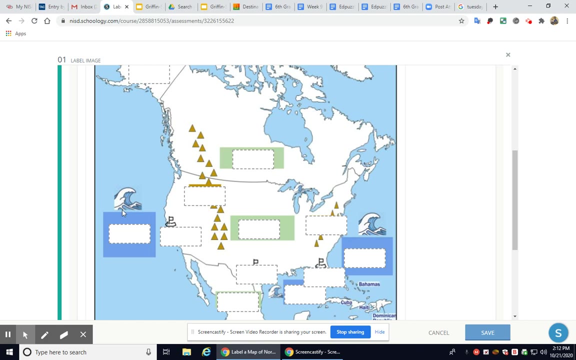 to the correct spot on the map in red. states are marked with a flag- okay, and bodies of water marked with a wave symbol. so, remember, the states are marked with a flag, all right, and the bodies of water we're focusing on is labeled with the waves- all right.